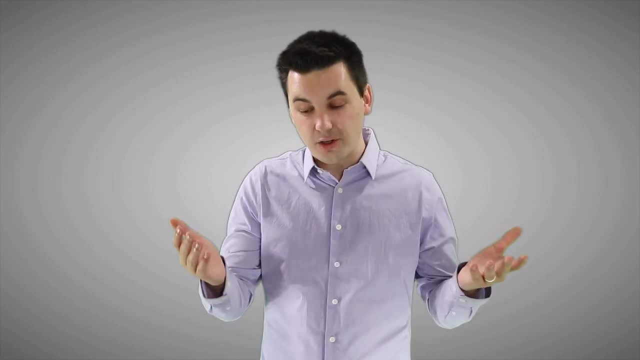 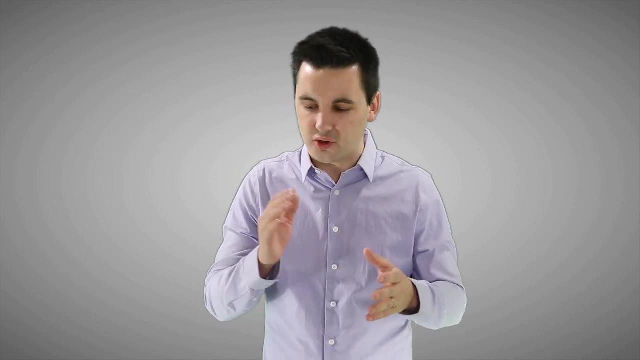 the world. As we continue to see countries trade with one another, we start to see them become interdependent on each other. What this means is these countries now rely, they depend on one another for different goods and services. In this unit, we're just talking about food and 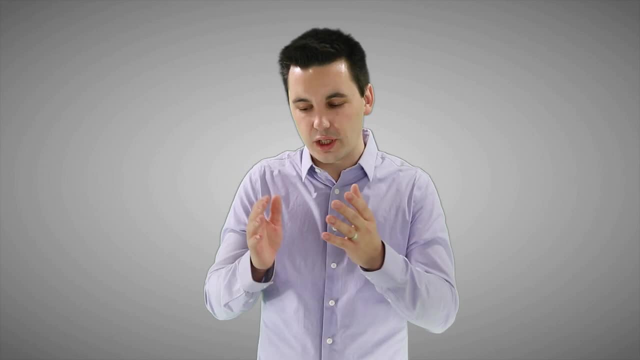 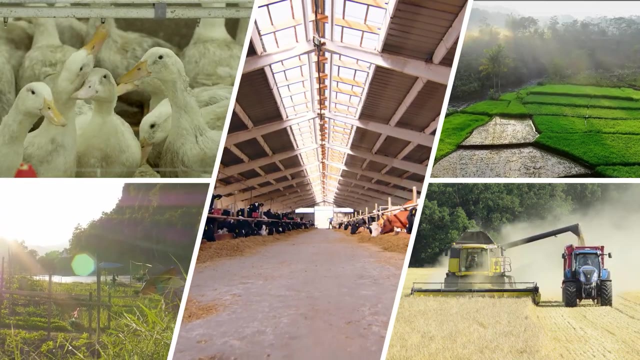 agricultural products. However, we can see this dependency when we get into our industrial unit as well. Countries around the world have distinct site and situation factors. They have unique climates and physical terrain that allows them to produce certain agricultural products, For example. we can see that countries around the world have distinct sites and situation factors. 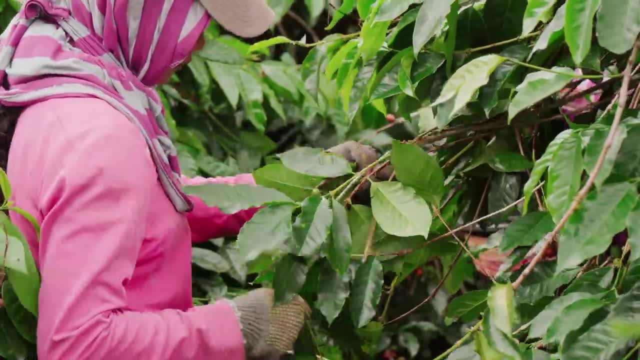 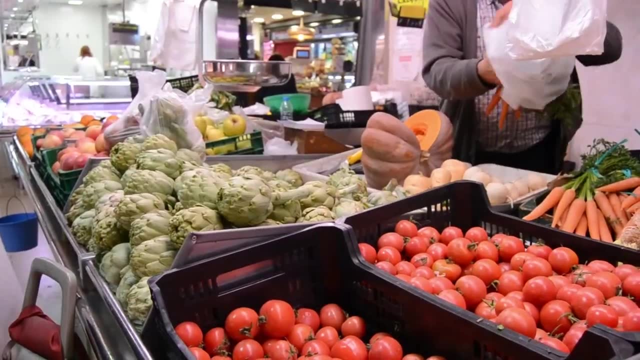 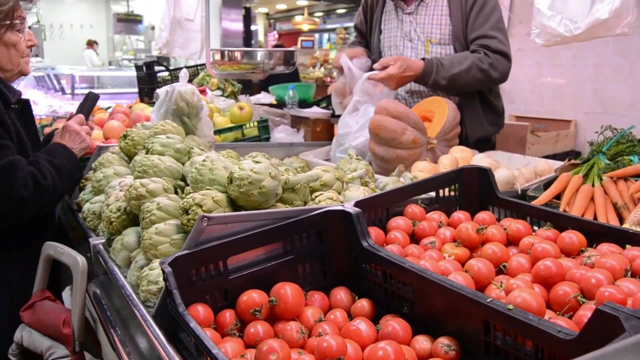 Countries in the southern hemisphere can produce a variety of agricultural products that the northern hemisphere countries can't. during the winter months, This allows our grocery stores to no longer have seasons, as countries can trade with other countries around the world to make sure they always have a variety of food. Today we can see that more developed. countries, or MDCs, benefit the most from our global trade of food. Oftentimes, food is produced in less developed countries and is shipped over to more developed countries. This allows the more developed countries to have cheaper food prices and also a larger variety of products. One of the 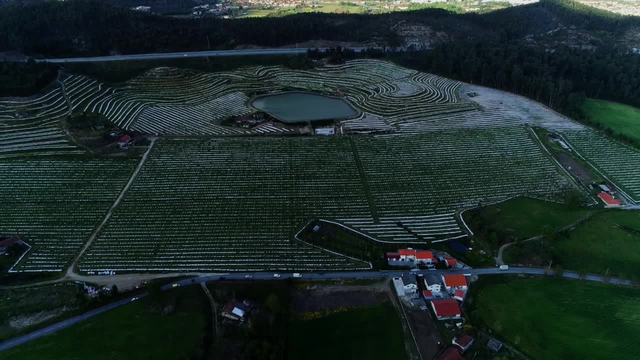 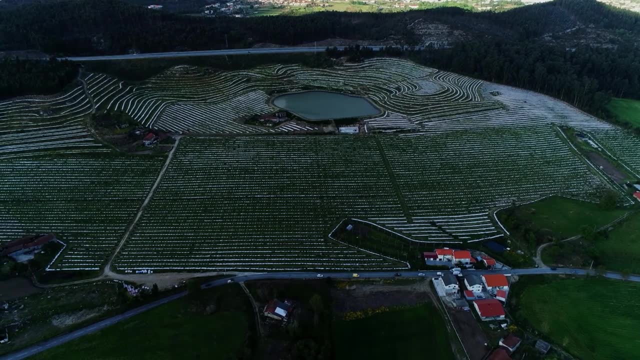 reasons we see farmers in LDCs export their agricultural products or luxury crops to more developed countries is because they're able to make more profit in those more developed countries. People in their own country can't afford to pay the higher prices. This creates an imbalance between 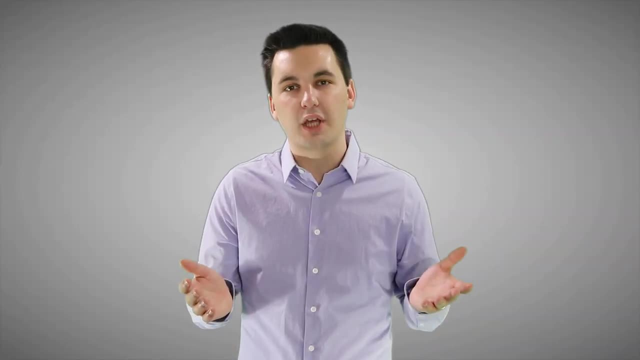 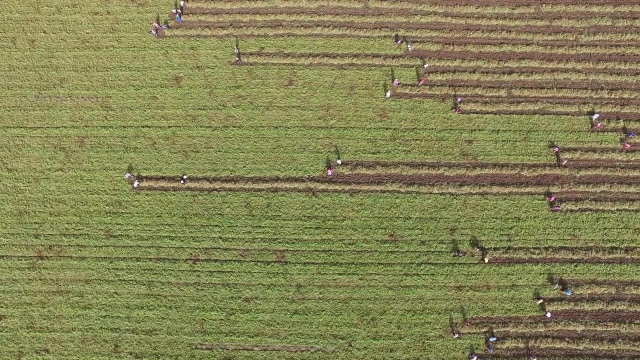 less developed countries and more developed countries. As farmers who are located in a less developed country now rely and depend on trade with a more developed country, farmers in LDCs' countries tend to think that more growth and development means more cost barriers that prevent. 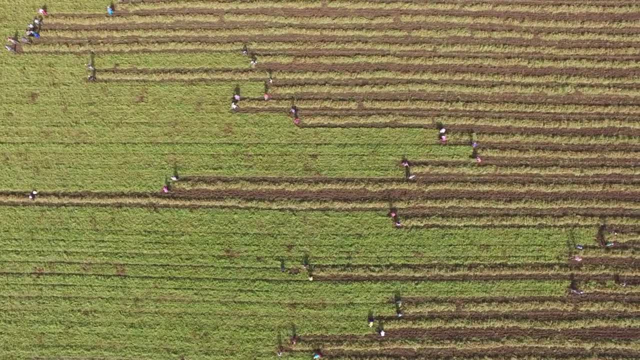 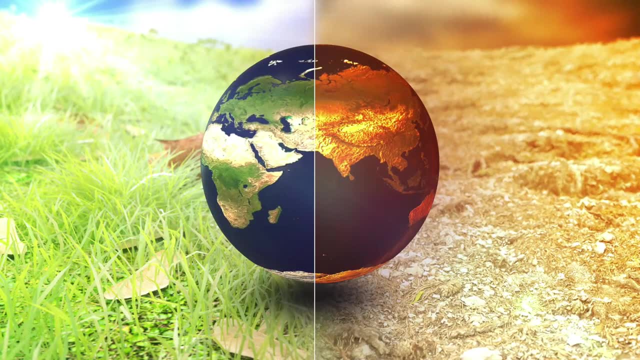 them from scaling up their business. They lack modern machinery and are more likely to exploit their natural environment to produce their crops. This can lead to deforestation, desertification, soil erosion and also the salinization of the soil. Salinization is when salt starts to build up. 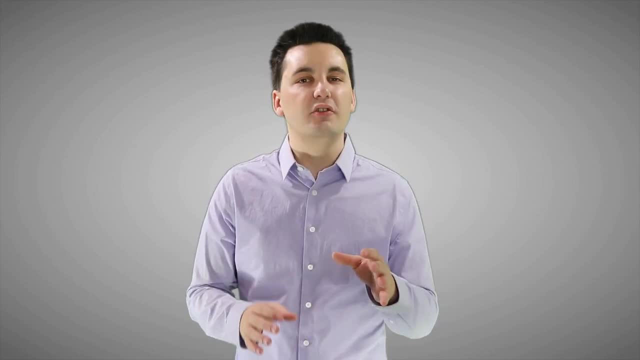 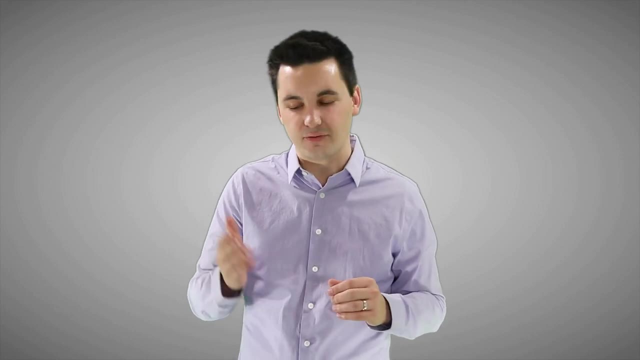 in the soil. This makes it difficult for plants to grow, as it prevents them from getting water. often happen due to the farmer's practices, such as monocropping, a concept we talked about in our Unit 5, Topic 6 video. 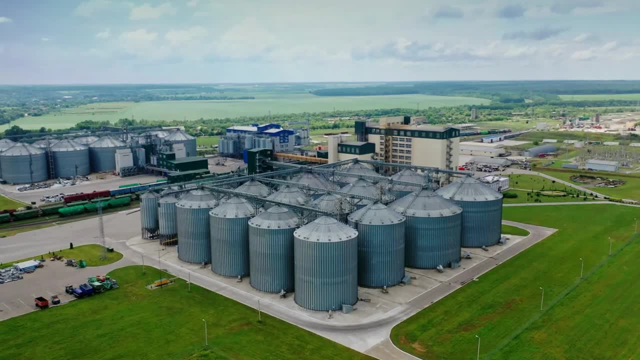 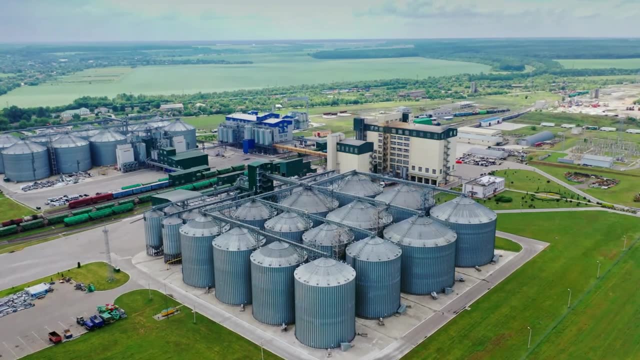 Now, farmers who are located in MDCs have a significant advantage over farmers located in LDCs, as they're more likely to receive subsidies from their government, which make it cheaper to grow their crops. More developed countries also have a more robust transportation system and infrastructure.